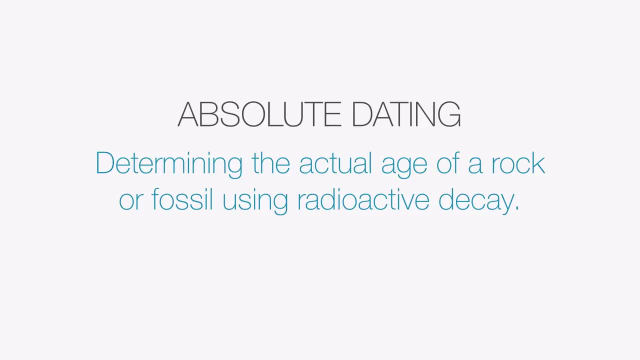 specific number. Now there's another type of dating that we use when we're looking at the history of the Earth, and that's called relative dating. Now this would be figuring out simply which rock or fossil or geologic event came first, which one came second, third, etc. 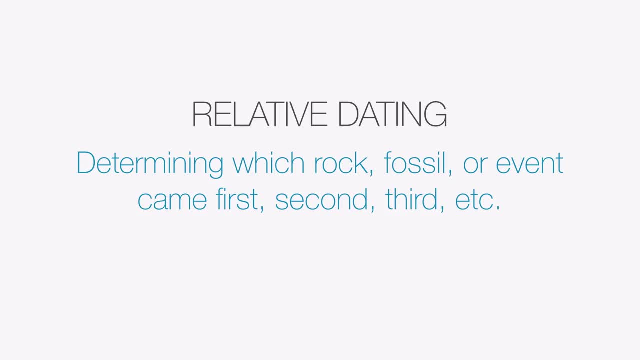 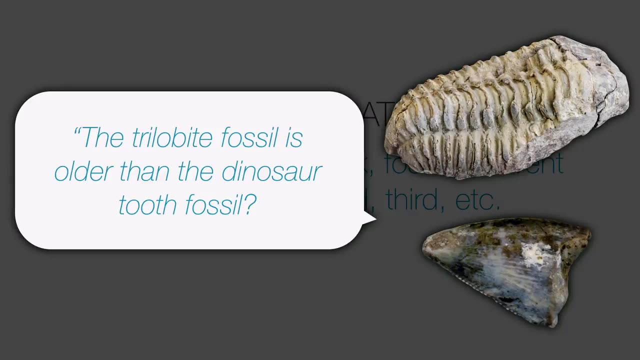 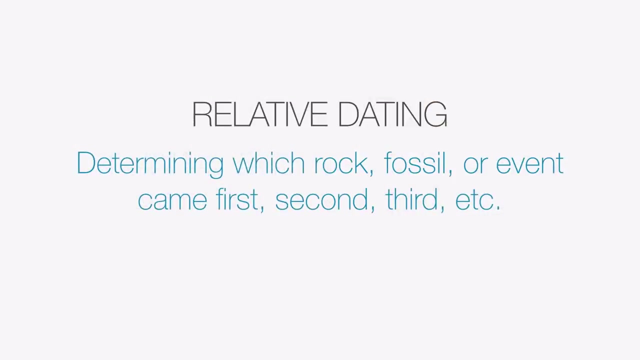 Without using any specific quantitative values. For example, if I were to say the trilobite fossil is older than the dinosaur tooth fossil, that would be an example of relative dating, because I'm not using any numbers, I'm doing a comparison. Let me give you one more example of the difference. 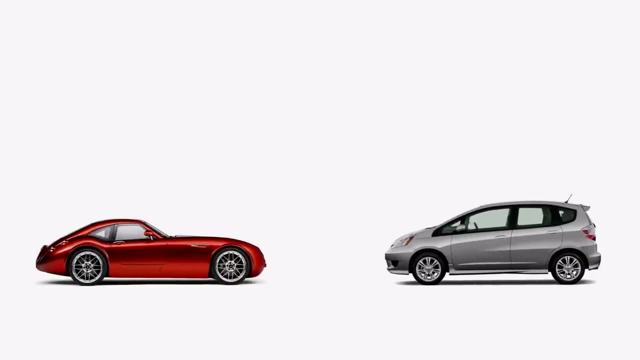 between absolute and relative dating. Let's take a look at these two cars here. What if I were to make a statement like: the red car costs $90,000 and the silver car costs $15,000?? Now, because I'm using specific numbers, this is an example of using an absolute comparison. 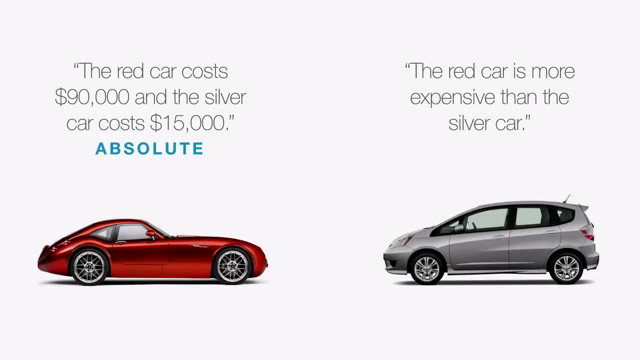 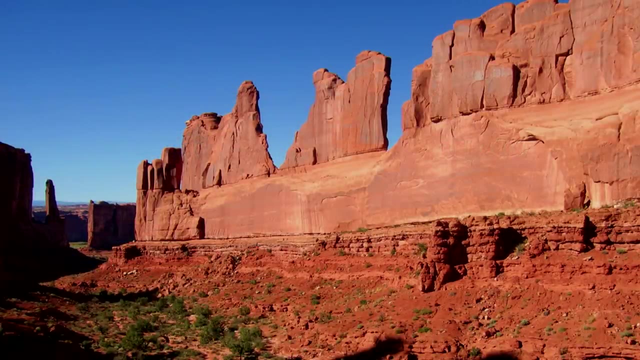 On the other hand, I can make a statement like: the red car is more expensive than the silver car. Now, because I'm not using any specifics, I'm simply doing a comparison. This would be an example of a relative comparison. What about in terms of rock layers? Well, here I have some layers of sandstone out in the American Southwest. 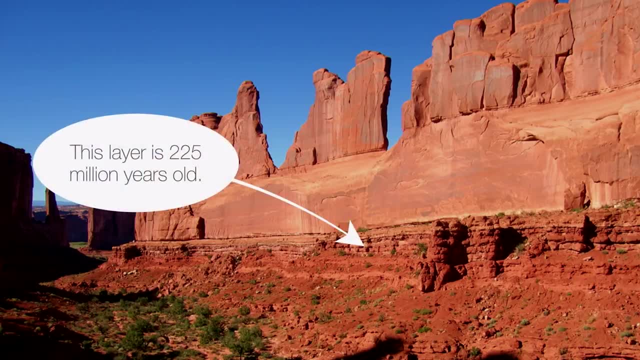 If I were to say something like this layer of rock is 225 million years old, that's an absolute dating statement, because I have a number, I'm being specific. But if I were to say this layer of sandstone is older than this layer, that would be an example of relative dating. Now, of course, in the study, 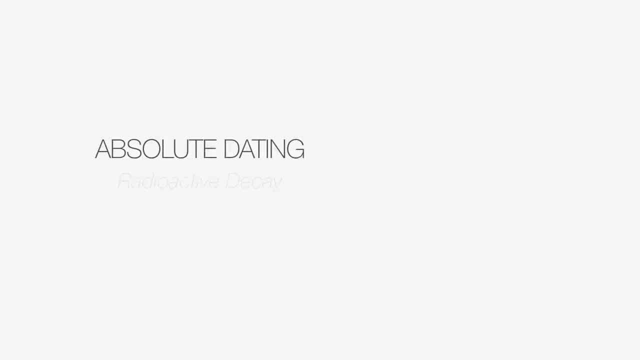 of Earth's history. we're going to use both absolute dating, through radioactive decay, and we're going to use relative dating, through geologic sequencing, And that's what I want to focus on today. So let's get into this a little bit. And before we get too deep, though, we have to start with one underlying principle, an assumption, if you will. 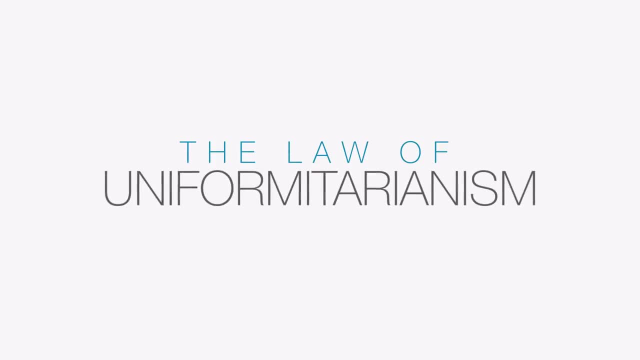 And it has a name. It's called the law of uniformitarianism. Yes, that's a nine-syllable word. Well, what this law essentially says is that all of the things that we observe happening on Earth today, including weather, storms and wind- 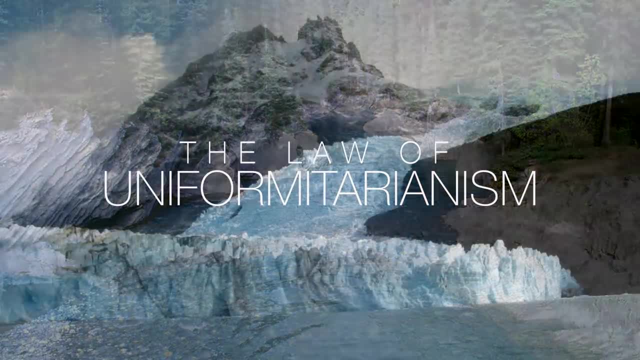 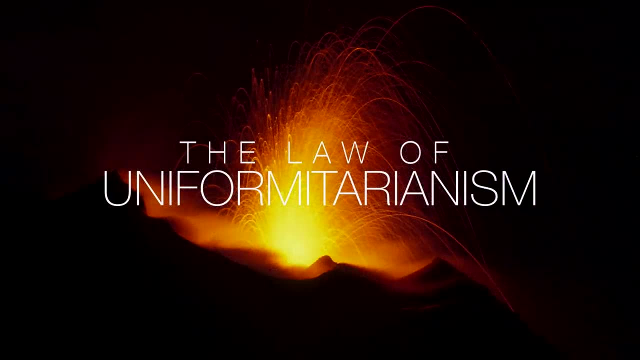 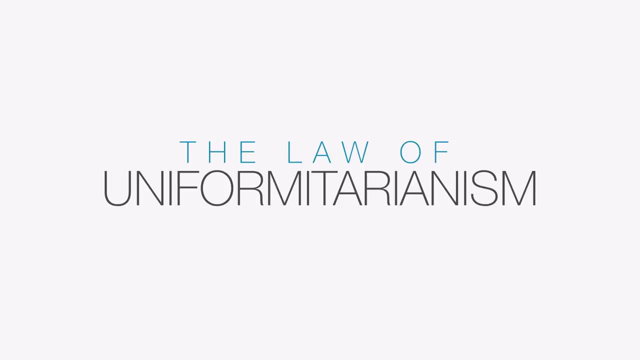 erosion and deposition by rivers and by glaciers, geologic events and tectonic events like earthquakes and volcanic eruptions and the motion of the plates- all of these processes that we see happening today. Well, the law of uniformitarianism says that we can assume that they happened the same way in the past. 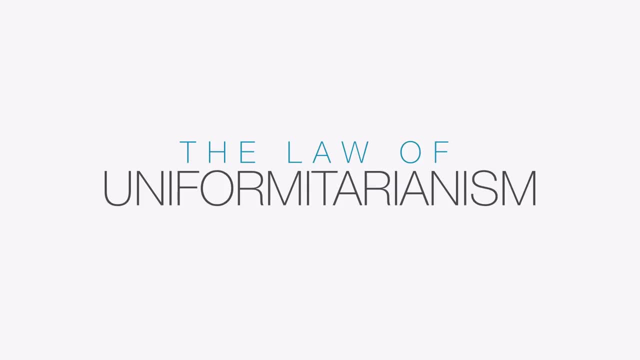 And that's an important assumption, because it allows us to look at rock layers from millions of years ago and have a good idea as to what actually happened to form those rock layers, because we're seeing the same types of things happening today. Now, one of the great tools we're going to use in studying the history of the path of the Earth, rather, is something called a road cut. 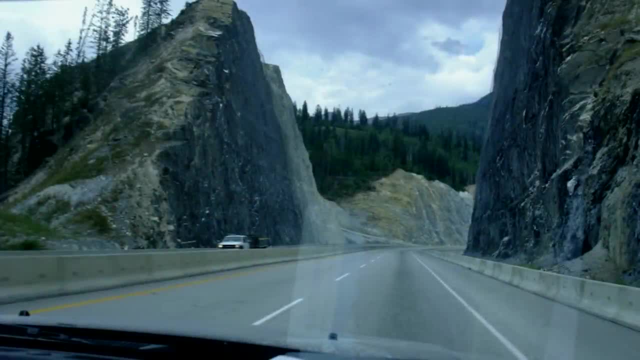 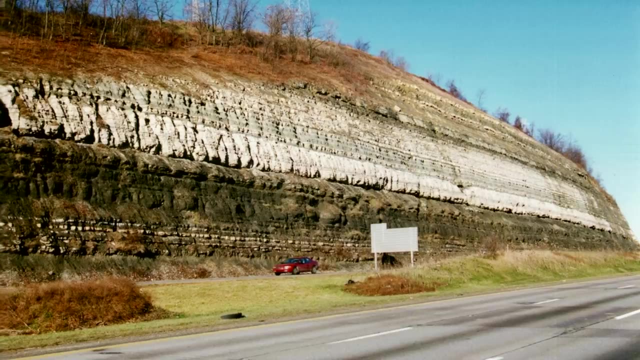 You see a road cut here. I'm sure you've seen it before. This is where rocks, mountains, are cut away by dynamite so that highways and roads could be built. Now what's great about a road cut is it allows us to see further and further back in time as you go deeper down. 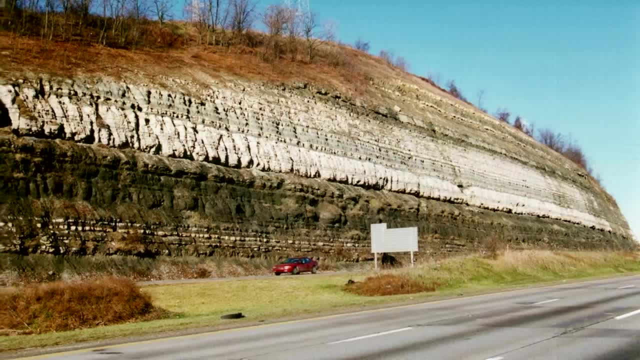